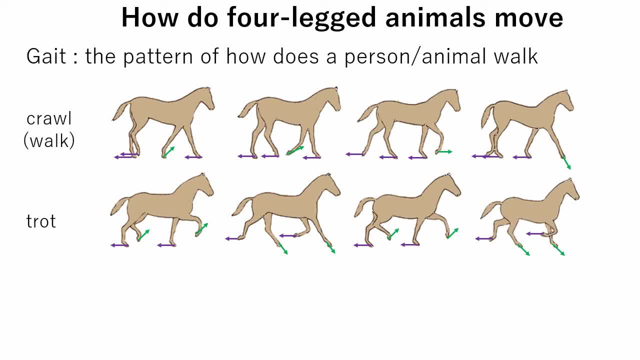 frequency of the legs being lifted and placed. the quicker, the less shaky it is. Stability is related to design of the feet as well. If the feet have a large area contacting with the ground, you will find it stand better while the other two legs are lifted. 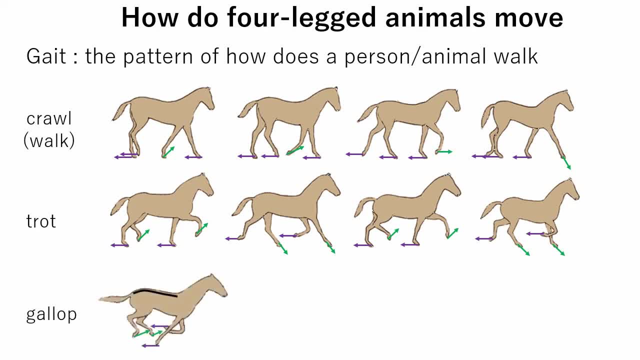 The gallop is the fastest gait. Each stride can cover more ground than in other gaits, but it's also very energy demanding. In the gallop we also see the greatest compressing and stretching of the trunk, with the tightest compression happening as the front limbs lift. 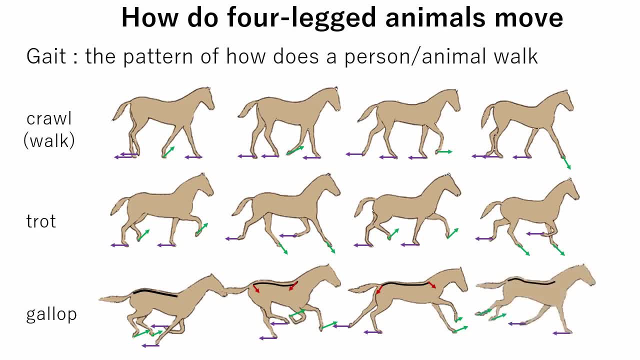 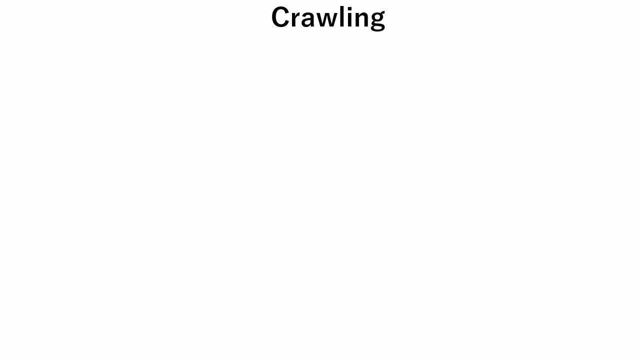 and the longest extension right before the front limbs land. In this tutorial for a quadruped robot, we will cover crawling and trotting. Now let's take a closer look at crawl gait. Crawling is a static, stable gait Inertial. 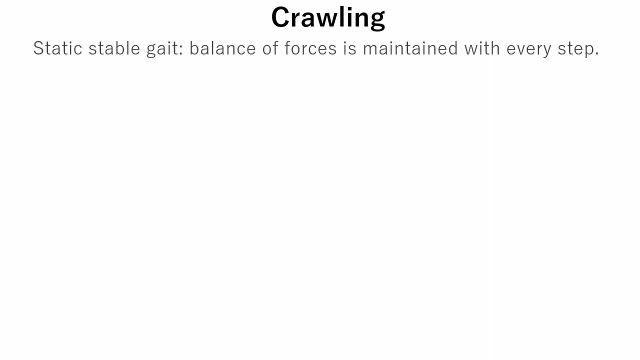 forces are negligible and balance of forces is maintained with each step. This means that the robot can stop at any time without falling. While crawling, the robot always has three points of contact with the ground. Also, the sum of moments around the line is the same. The robot can stop at any time without falling. While crawling, the robot always. 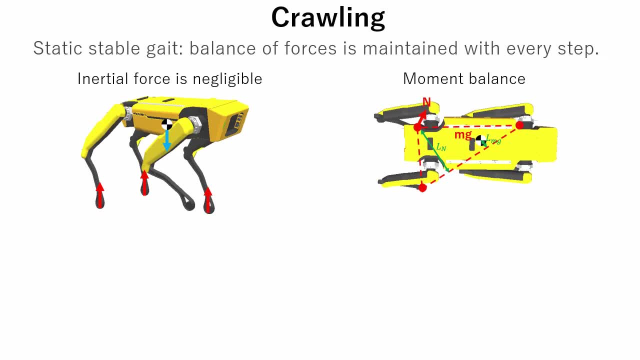 has three points of contact with the ground. Also, the sum of moments around the line connecting two diagonal contact points with the ground should be more than zero. In other words, the center of mass should always be inside the triangle of ground contact points. 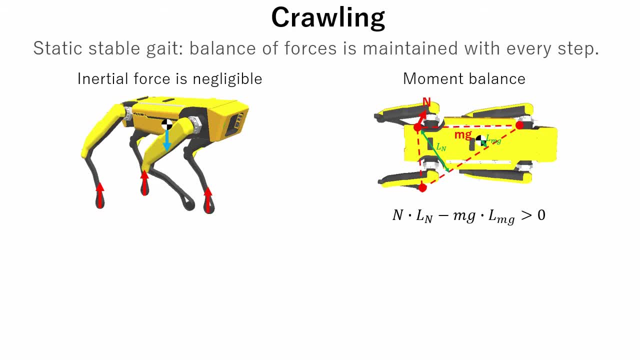 Otherwise, as soon as the robot raises its leg, the robot will fall. Let's take a look at the gait sequence. When the robot raises legs on the left side, it leans a little bit on the right side to move its center of mass, and vice versa. Note that the 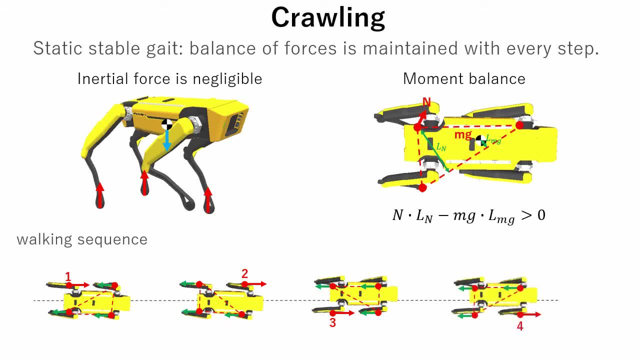 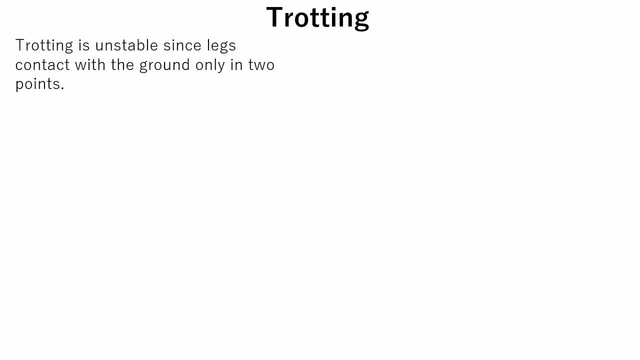 amount of how much the robot leans aside can be changed in the gait controller by body shift y parameter. Now let's talk about trotting, As it was mentioned before. trotting is unstable since legs contact with the ground only at two points at the same time. So some kind of stabilization. 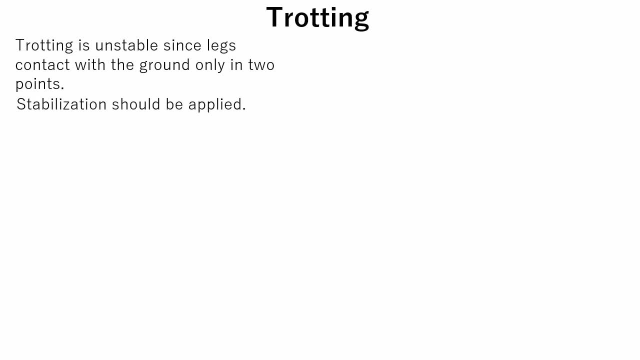 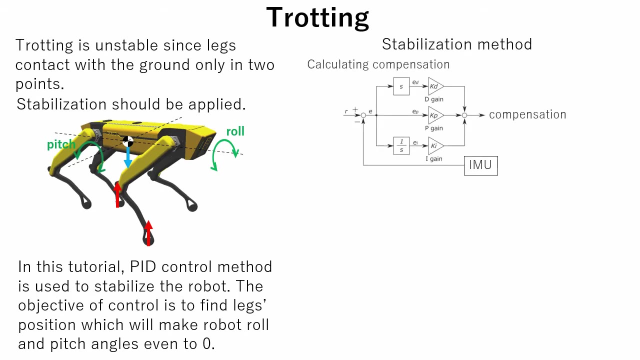 control should be applied to stabilize the robot. The objective of control is to find the position of the legs which will make robot roll and pitch angles even to zero. In this tutorial, PID control is used to stabilize the robot. This is how compensation is calculated. R stands for the objective values of pitch in roll. 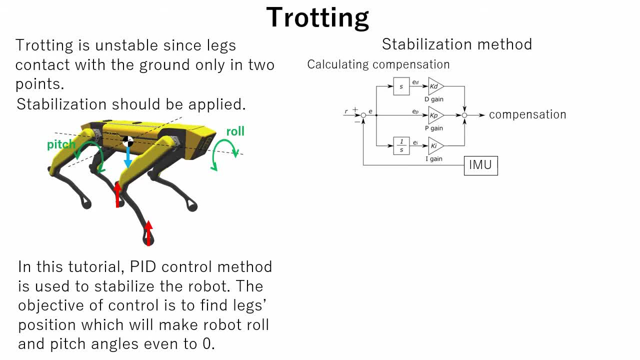 that is zero. E is the difference of the objective values in data obtained from the IMU. Since this is a discrete system, to calculate differential part we divide the difference of current and previous error values by current time step value. To calculate the integration part, we add a product of current time step and. 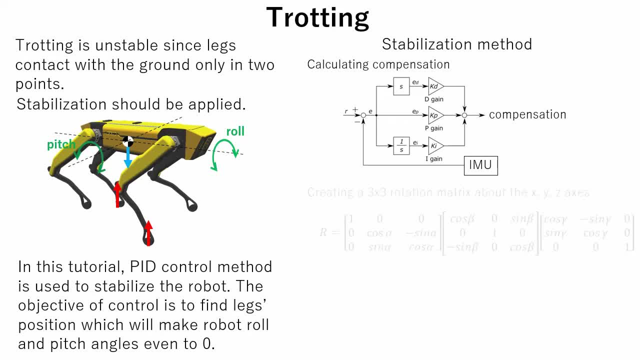 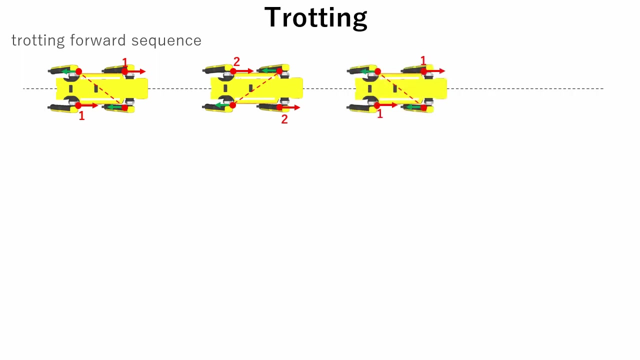 current error value to the previous integration value. Then rotation matrix about each axis is calculated. Finally, corrected leg position is calculated using rotation matrix and leg positions calculated from trot sequence. This is trotting forward sequence: While two diagonal legs swing forward, the other two legs kick the ground. 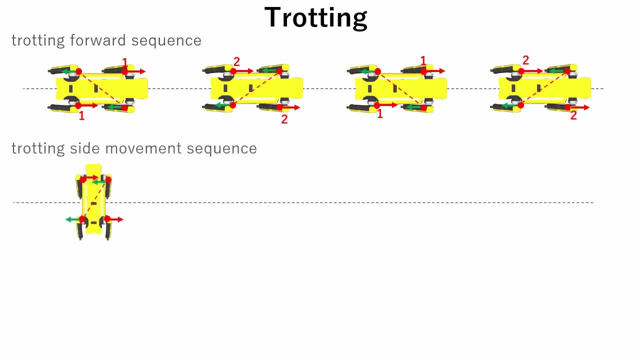 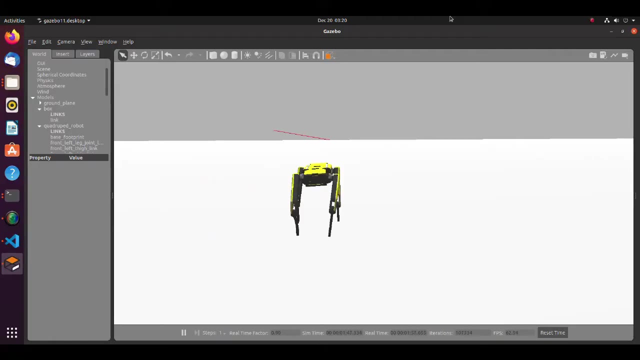 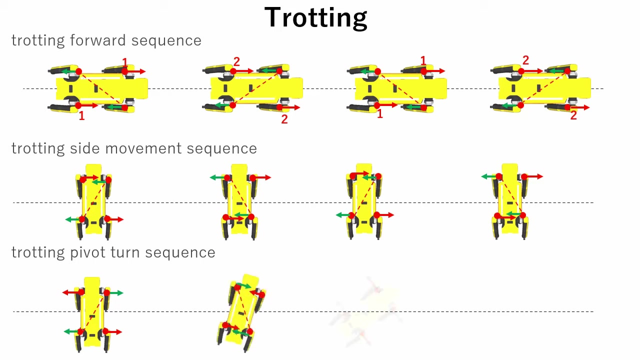 For side movement the idea is the same. Note that diagonal legs always swing to the robot moving direction and kick to the opposite direction. For the pivot turn we have a different situation Here. two diagonal legs move in directions opposite to each other to create a momentum which rotates the robot. 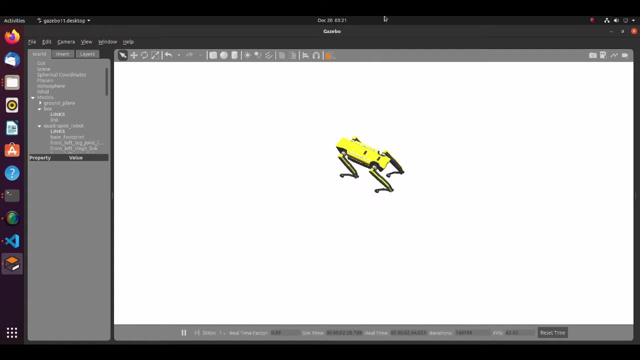 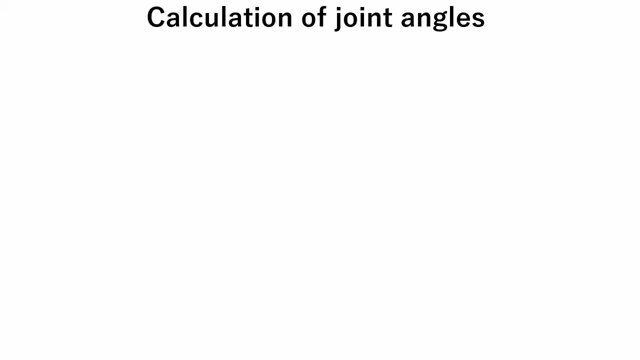 Overall. the higher frequency of the legs being lifted and placed, the less shaky robot movements become. But if the leg's movement speed exceeds the actuator limit, it will result in divergence of the control. In this part we will talk about how to find joint angles of the leg. 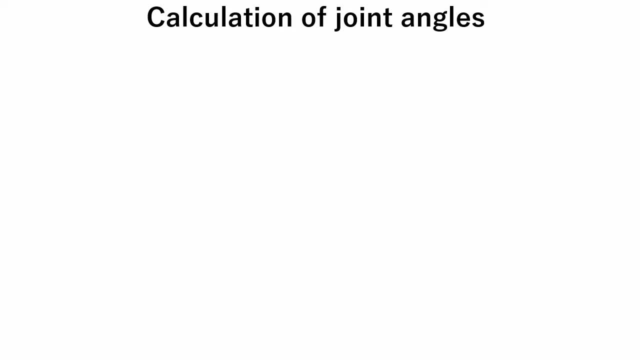 Usually this is done by inversion. This is done by inverse kinematics. calculation For inverse kinematics: please check this tutorial. But in this tutorial, as an alternative solution, we will find joint angles trigonometrically. This is a leg. The coordinate origin is the rotation center of the joint which connects body and the thigh. 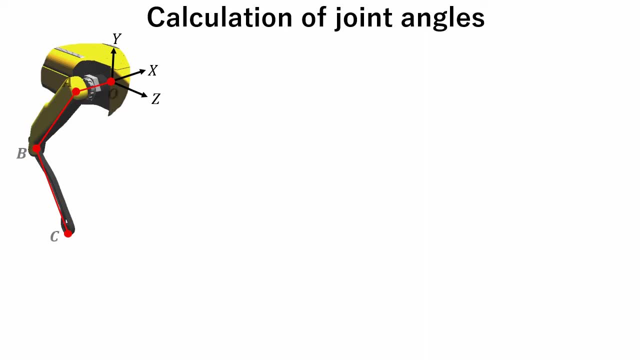 Each part of the leg is simplified as a link. The origin is O and this is also rotation center of the first link. We have two more rotation joints at points A and B. Point C is the contact point of the leg and ground. Each link length is set as L1, L2 and L3 respectively. 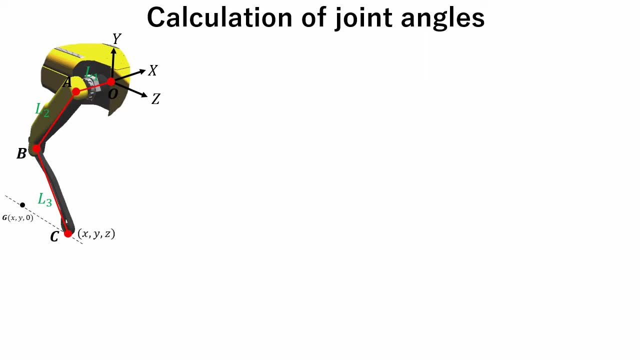 Also, we set point G, which is on the XY plane and has the same XY coordinates with the point C. OG is the distance between the origin and leg contact point. in the XY plane. OG can be found with the next formula: OA and AG are vertical to each other. 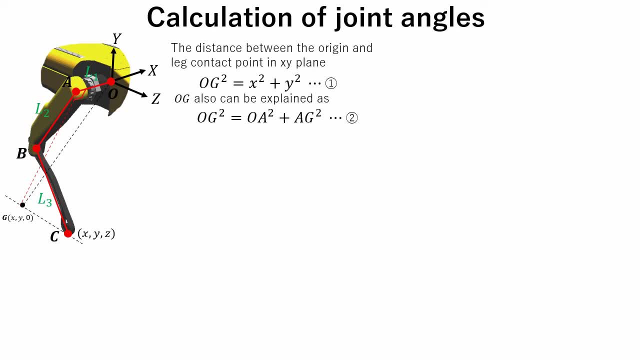 So OG also can be explained as this formula. Using formula 1 and 2,, the following equation is derived: AG is expressed as shown For the later calculations. we also have to find length of AC. Since AG and GC are vertical to each other, AC is expressed like this: 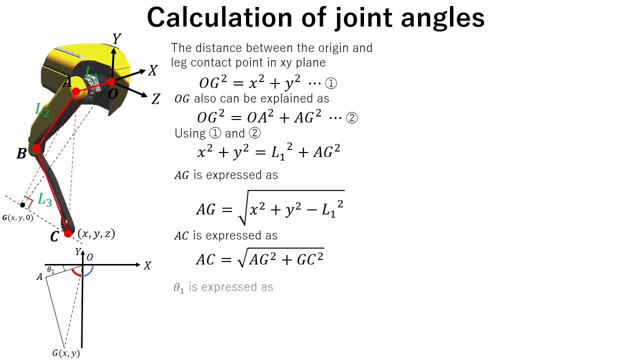 Now let's find out theta1.. As shown on this figure, theta1 can be found subtracting red and blue angles from pi. So theta1 can be expressed like this: Note that this formula may differ depending on how you set your coordinate system, but the idea remains the same. 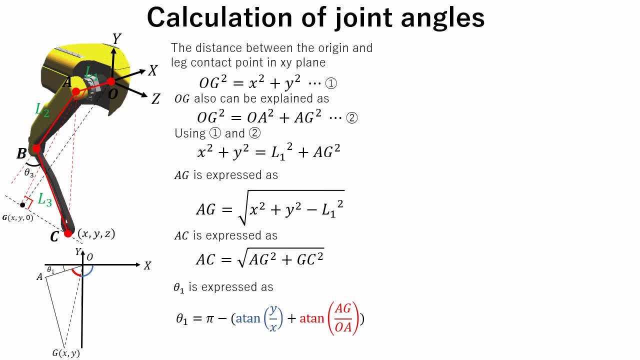 Now we are going to find out theta3.. Theta3 can be found out by subtracting angle alpha from pi. Using the law of cosines, we obtain the next formula Transforming this equation in respect to alpha. Alpha is expressed like this: 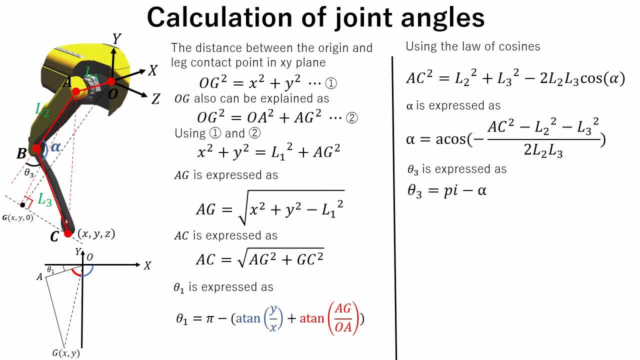 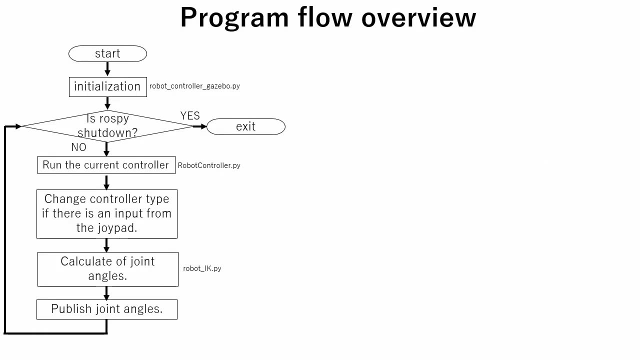 So theta3 can be obtained by subtracting alpha from pi. Theta2 can be found out by subtracting the red angle from the blue angle, like it is shown in this figure. Note that all these angles are on the same plane. Here is the rough program flow. 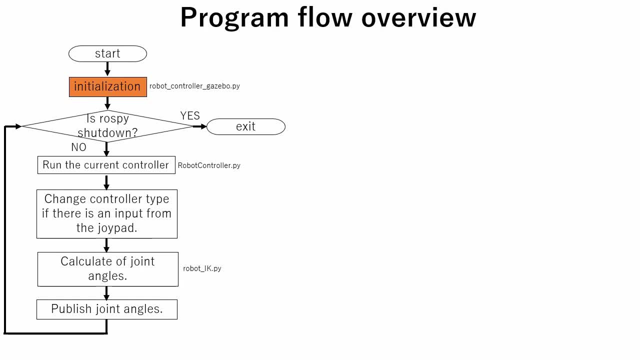 In initialization state, robot dimensions and controller initializations are done Here. we also subscribe to joypad and imu topics and set publishers for each leg joint. This robot has three operation modes: Crawl, trot and stand. Depending on in which operation mode the robot is, an appropriate controller is selected.